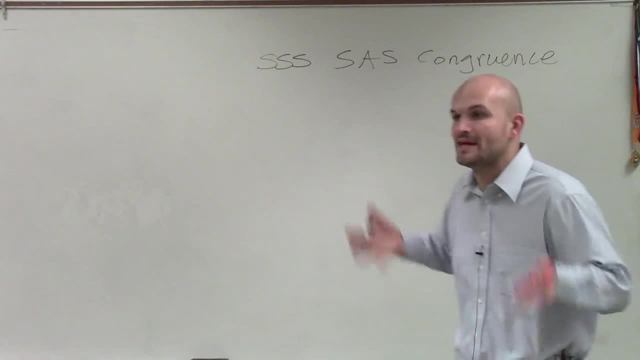 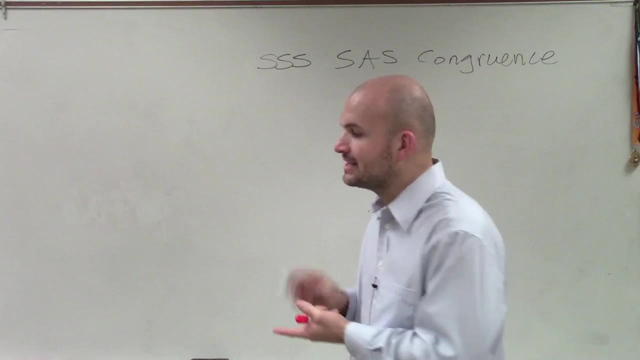 So what we're going to do for this one is now: we want to be able to show that two triangles are congruent, And if two triangles are congruent, that means their angle measure is exactly the same and the lengths of their sides are exactly the same. 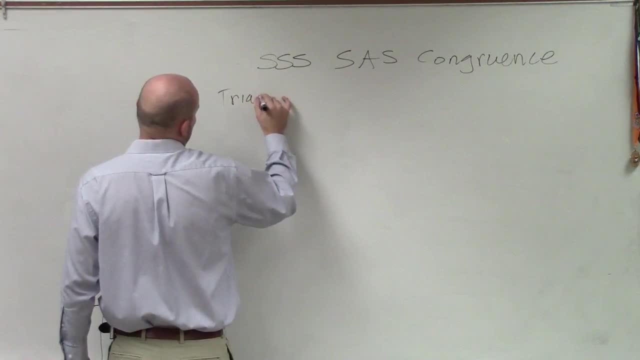 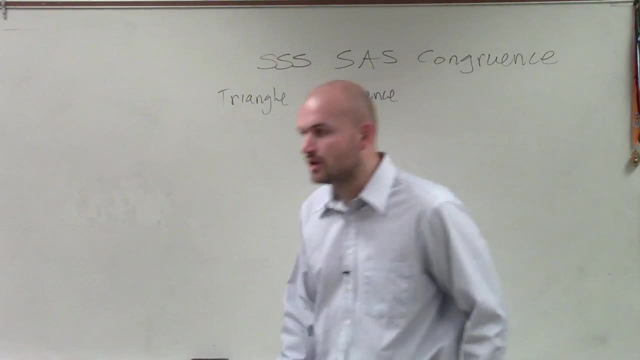 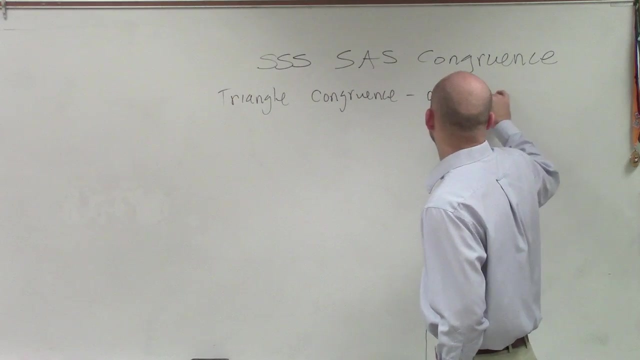 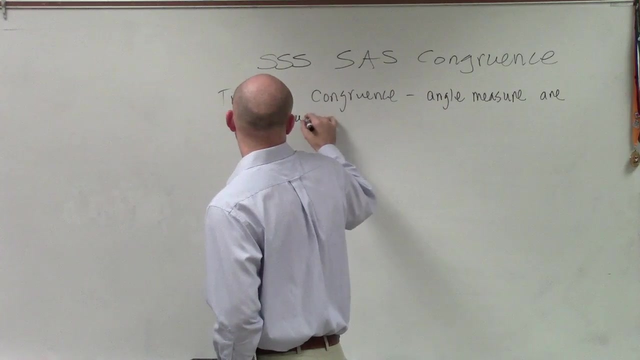 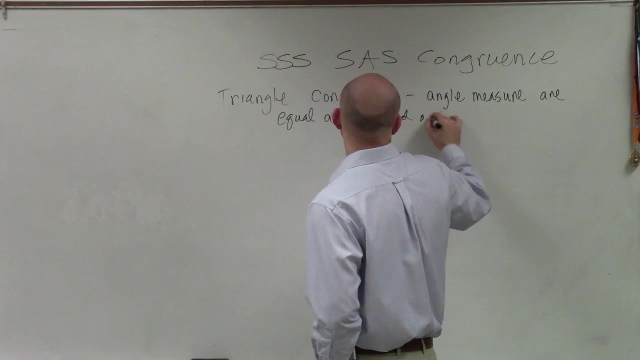 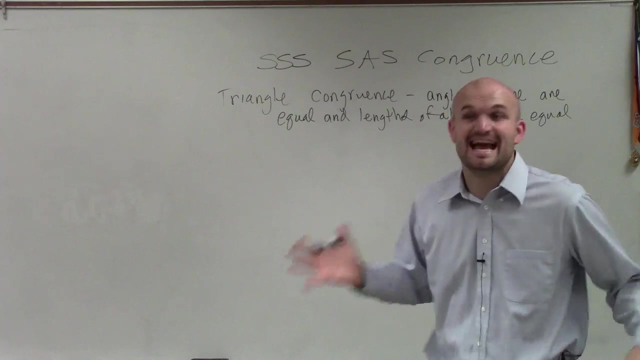 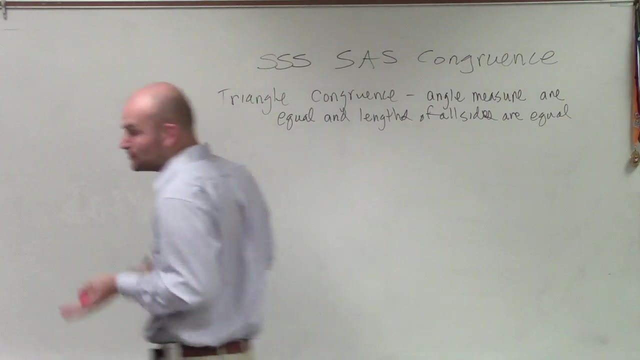 All right, So let's write that down, Please. If you have two triangles that are congruent, therefore they have the same measure and the lengths of all sides are equal. That means everything is exactly the same with both triangles. exactly the same. 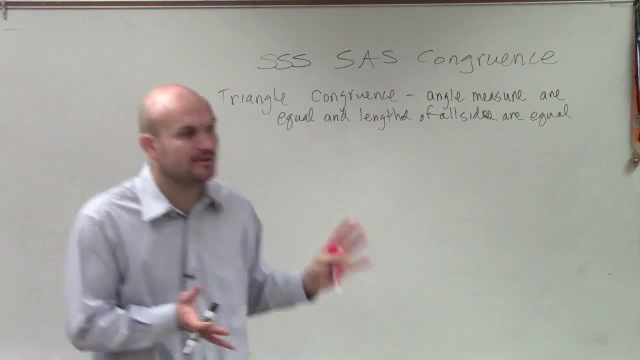 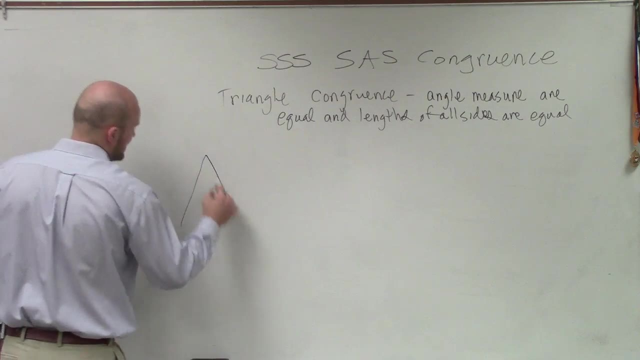 Every angle is equal to every angle and every side is equal to every side. All right, So there's going to be two ways that we're going to be able to show that triangles are congruent, And the first way is what we have side, side, side, which we call SSS. 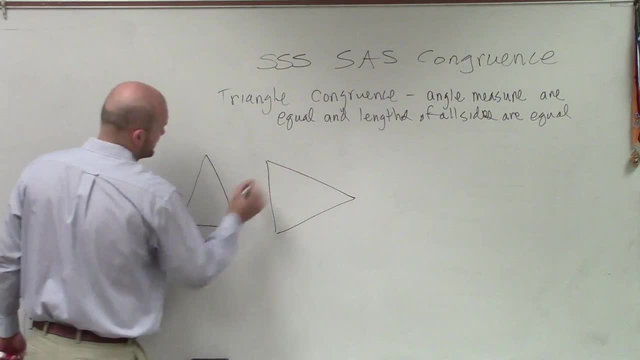 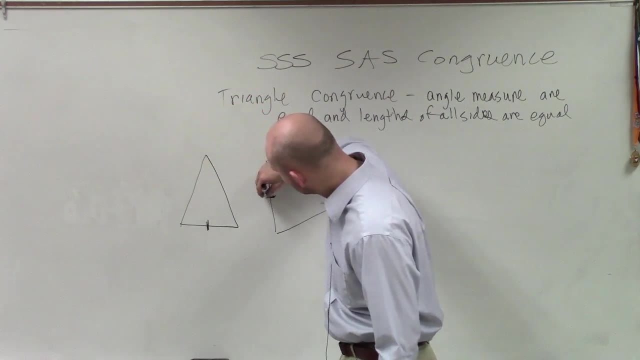 All right. And what SSS is going to tell us is, if we have two triangles, All right. Now remember when we apply these little tick marks. if you guys remember, when we were talking about an isosceles triangle, I would give two angles a little tick mark. 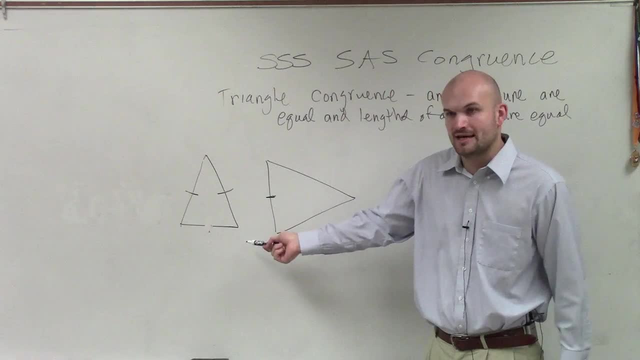 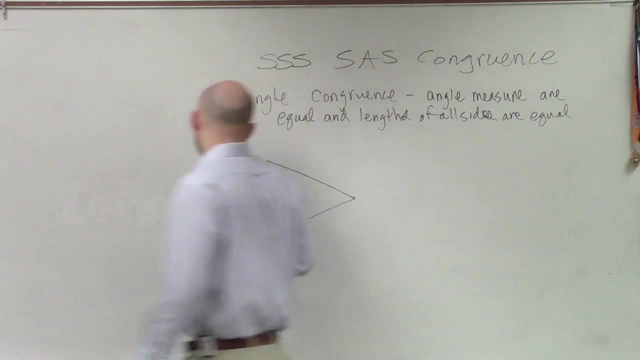 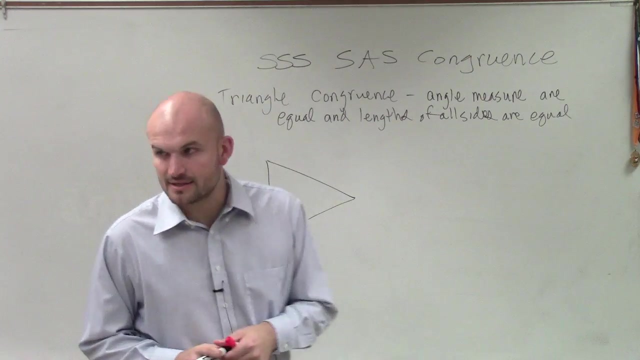 like that right. What that meant is that length is equal to that length, Correct? Yes, That's why we applied the tick marks: That length is equal to that length. So if I have on these two triangles, I say that length is equal to that length, what that is telling you? 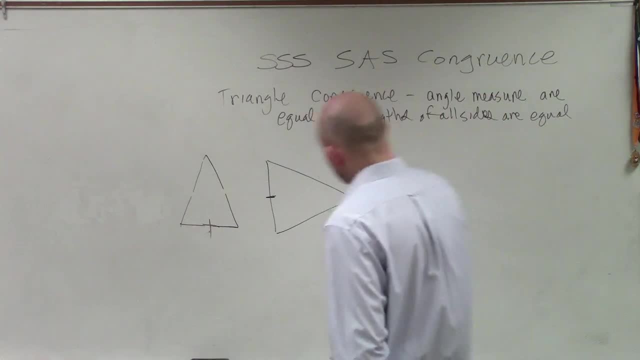 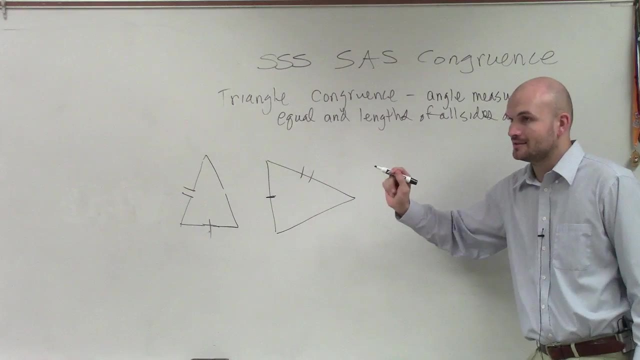 is that side is equal to that side. And then if I give this one two tick marks and that one two tick marks, what that is telling you is that side is equal to that side. And on the third one, if I have three tick marks here, 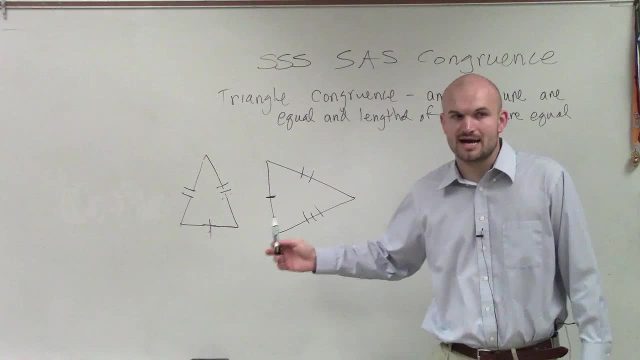 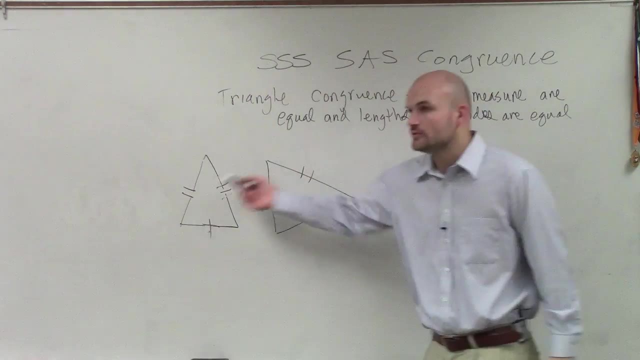 and three tick marks there. that's telling you that side is equal to that side. And, ladies and gentlemen, when we have all three sides equal to all three sides, you guys can see this is what we call side, side, side. Each side is congruent to the other side. 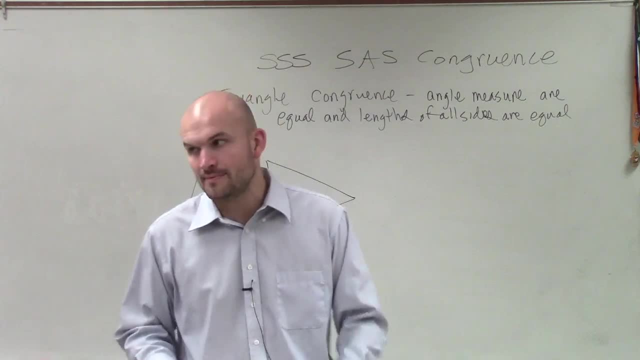 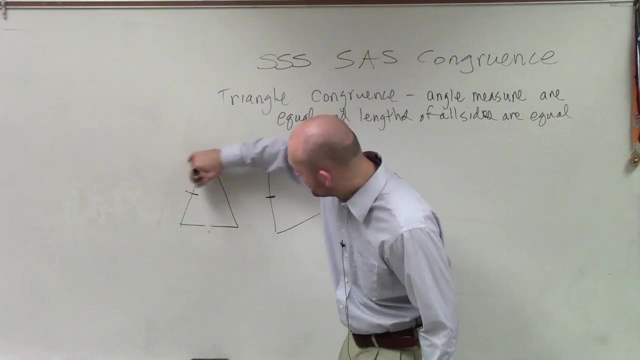 Is going to tell us is, if we have two triangles, all right. Now, remember when we apply these little tick marks. if you guys remember when we were talking about an isosceles triangle, I would give, like two angles a little tick mark, like that right. What that meant is: 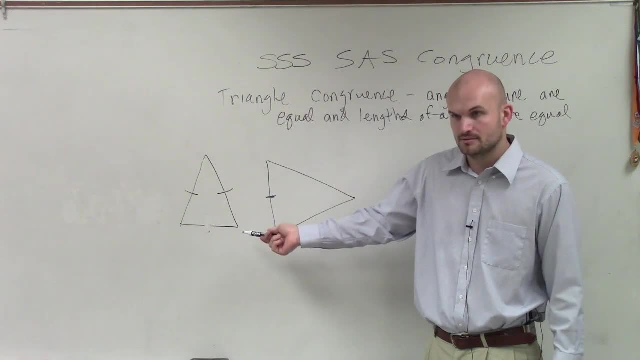 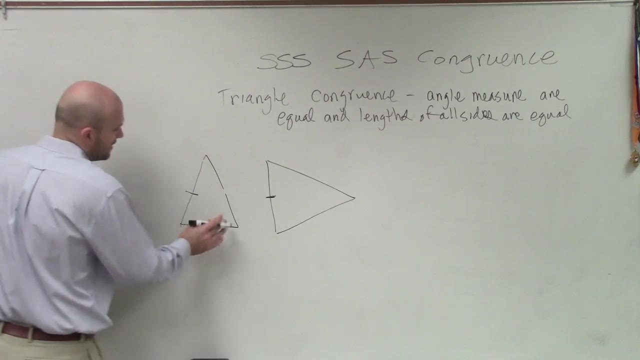 that length is equal to that length, Correct? Yes, That's why we applied the tick marks: That length is equal to that length. So if I have on these two triangles, I say that length is equal to that length And that think is. 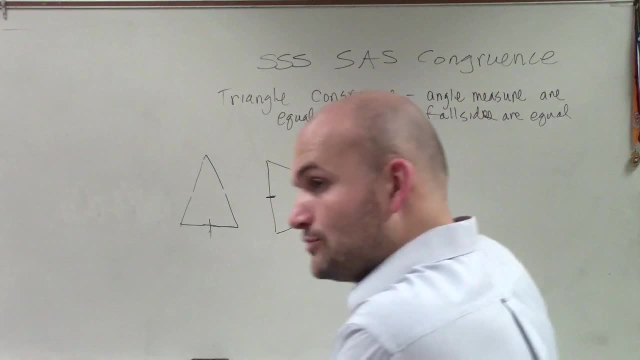 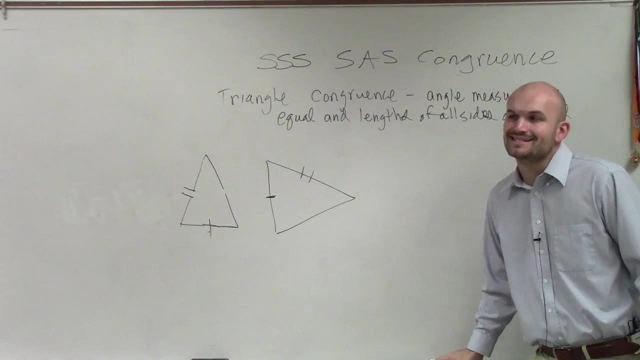 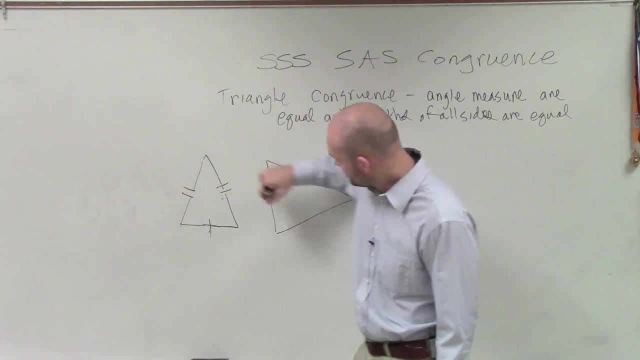 What that is telling you is that side is equal to that side. And then, if I give this one two tick marks and that one two tick marks, What that is telling you is that side is equal to that side. And now on the third one, if I have three tick marks here and three tick, 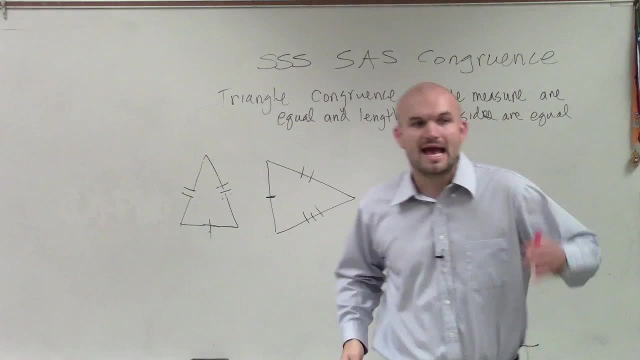 marks there, that's telling you that side is equal to that side. And, ladies and gentlemen, when we have all three sides equal to forward, But if that's the left side, it's going to show us that left side is equal to the right. 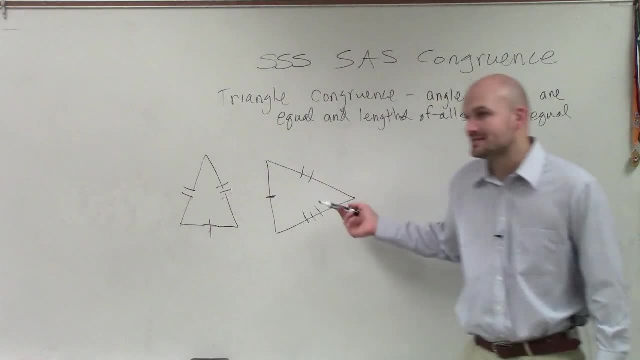 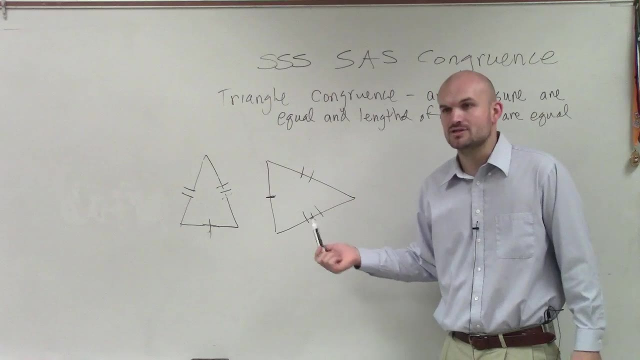 side, double-edged triangle. All right. So with that in mind, this actually oli language is to all three sides. you guys can see this is what we call side side side. Each side is congruent to the other side. So guess what? These two triangles are congruent in measure. 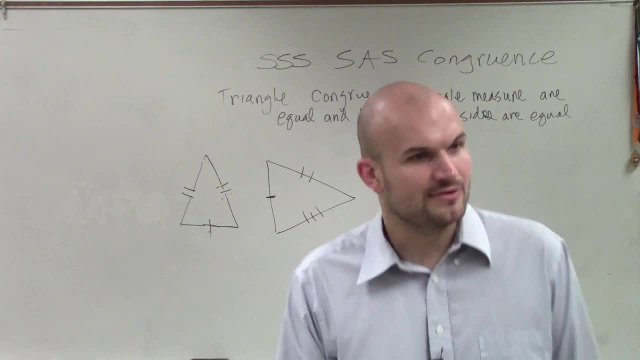 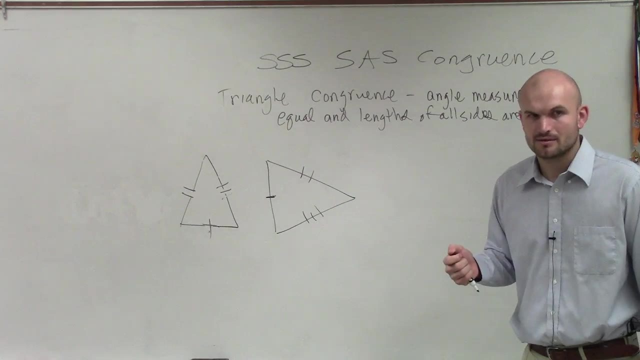 If they're congruent in measure because their sides are equal. what do you think that tells us about their angles, Alex? What do you think their angles are? Do you think their angles are going to be equal in measure? Yeah, they will be All right. The next one, So this. 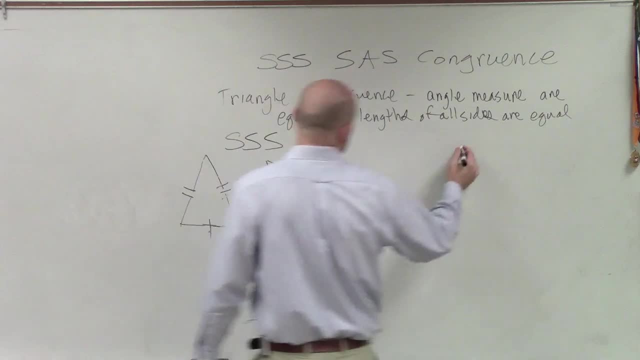 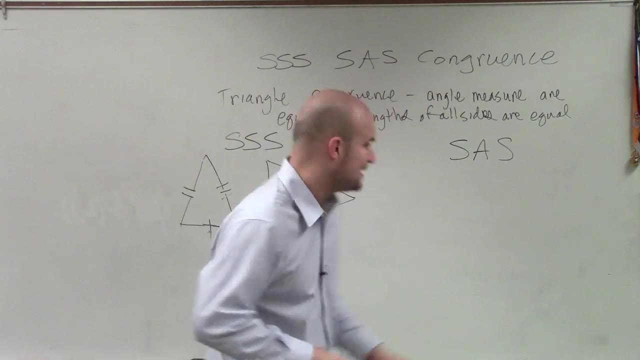 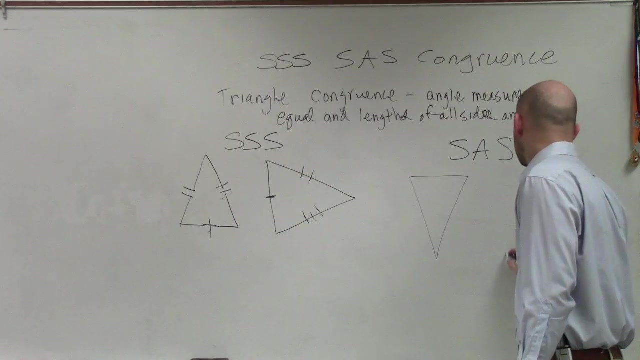 is what we call side side side. The next one is side angle side. OK, When you guys are looking at side angle side, what we have for that, when doing side angle side, what we have to have is we have to have sides that are equal in measure, but then we also 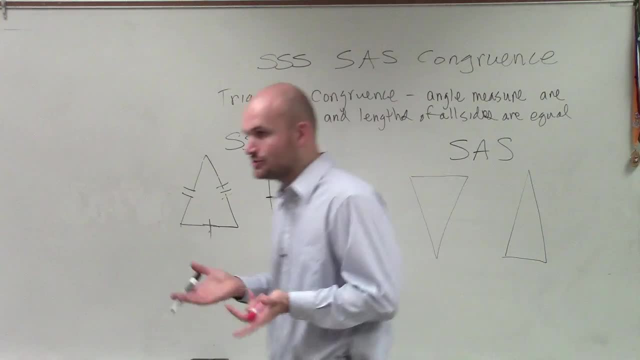 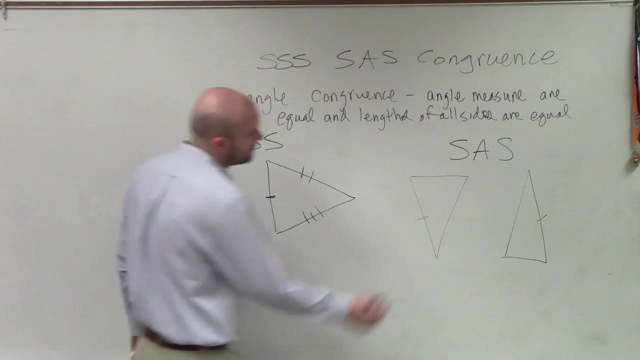 have to have an angle that is in between our two sides. So let's say we have: these two sides are equal in measure. These two sides are equal in measure For it to be side angle side. listen to how I say it: Side to angle to side.